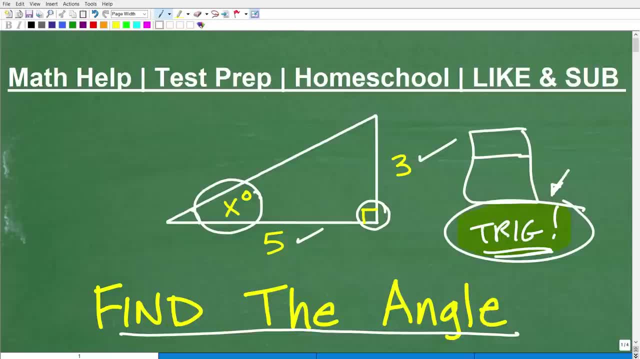 is John. I'm the founder of TC Math Academy. I'm also a middle and high school math teacher. I've been teaching math for decades And I'm telling you right now: if you're struggling in math, don't give up. You can do much, much better. but it requires two things. One: you do have to. 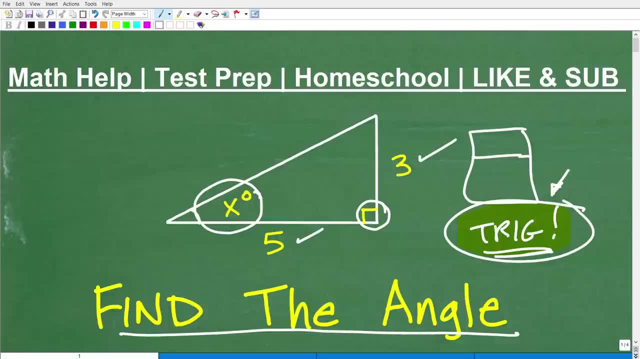 work hard to learn mathematics, So work harder. The second thing you need is great math instruction, clear and understandable. So if you're at the middle school, high school or even college level, check out my Math Help program. You'll find a link to it in the description of this video. 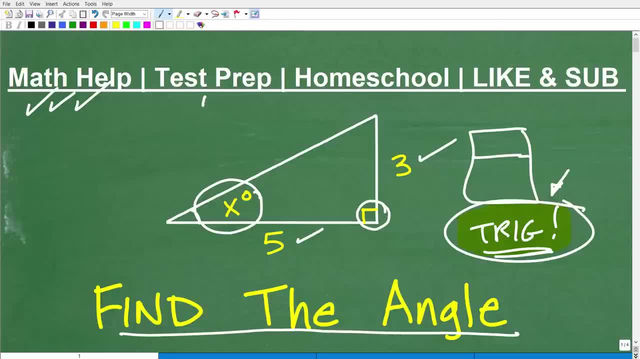 I can help you out big, big time, I promise. Also, if you're preparing for any sort of test that has a math section- things like the GED, SAT, ACT, ASVAB, maybe a teacher certification exam- I have a ton of test prep courses that can help you study for those exams. If you homeschool, 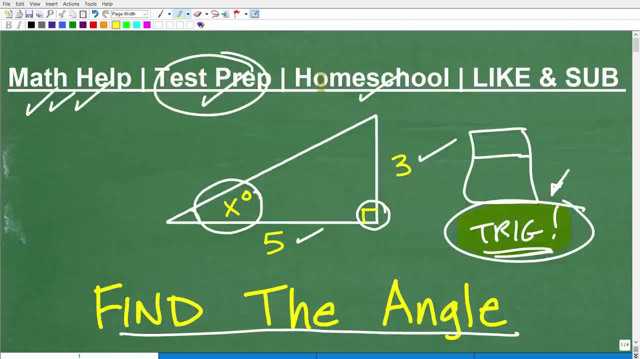 I have excellent middle and high school math courses for homeschoolers And if this video helps you out, help me out by liking it and subscribing to my channel. But let's go ahead and get into some basic right angle trigonometry. So if you've never seen trigonometry in 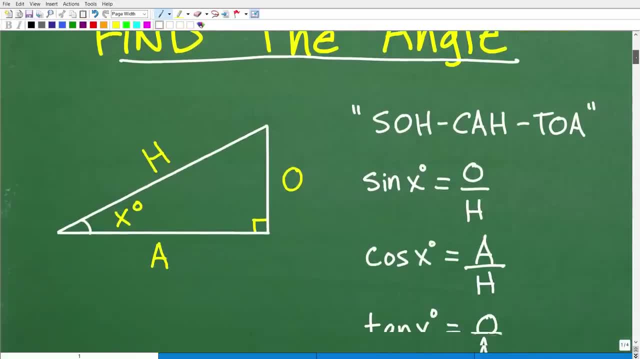 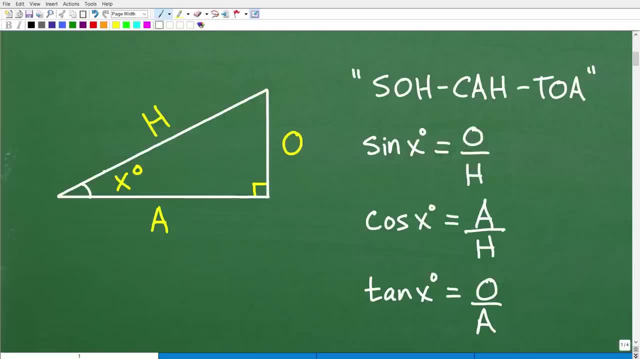 action. well, you're going to learn something right now, Okay, All right, So let's get to it And first things first. So here is our triangle, but you can see I have it replaced with- I took the sides out and I have O, A and H, So I'm going to get to this here in 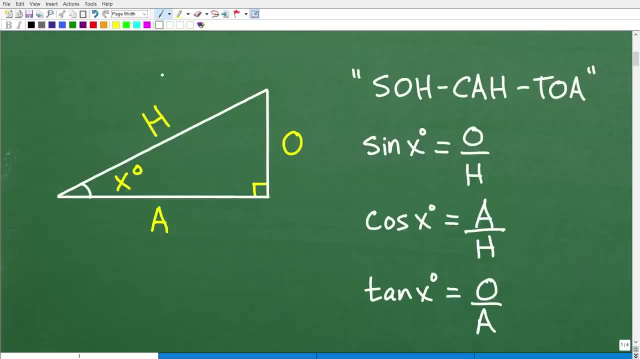 just one second. but let's just look at this triangle, And at first we have some abbreviations. Let's talk about what these abbreviations mean. So here is our angle: X degree. We're trying to figure out What is the angle measure of this angle, right? So we know that this is 90 degrees. And then 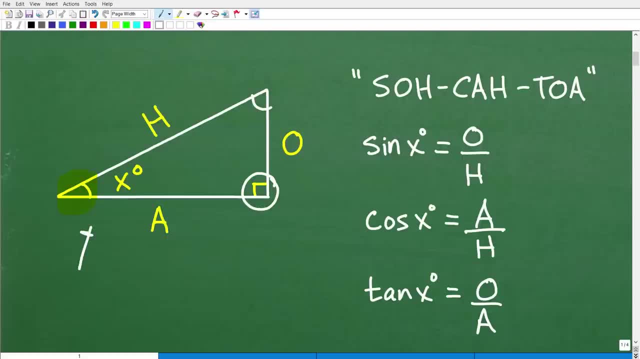 you have another angle over here And then we have an angle here. Our focus is on this angle right there. So when you're looking at an angle in a particular triangle, a right triangle right here, the side that's right next to the angle, that's forming the angle. 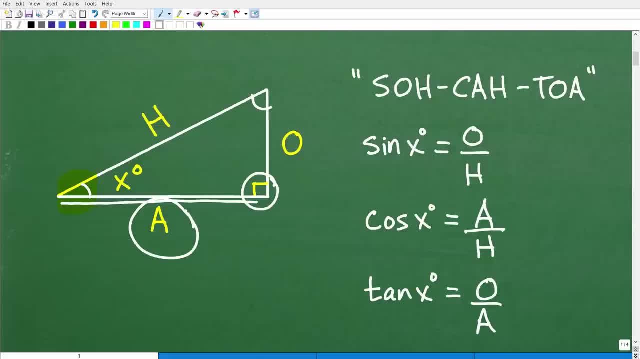 this one right here is called the adjacent side. So we have an A right there Now in a right triangle, the longest side of any right triangle, uh, we refer to as a hypotenuse. It's always opposite of that right angle. So this side right here is the hypotenuse, This side here is the adjacent. 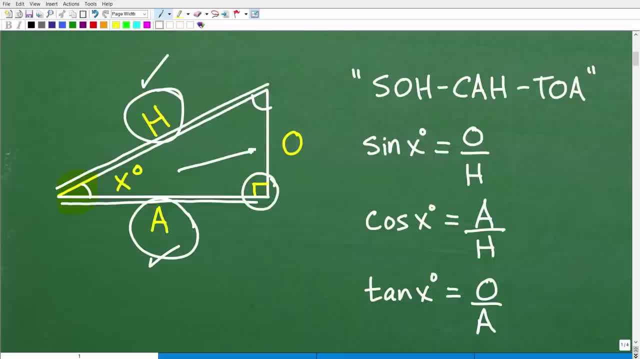 because it is next to the actual angle And then this side over here is opposite. It's the opposite away from the angle. So when we're looking at these um sides of a right triangle, we have to look at it in terms of this particular angle. So this angle right. 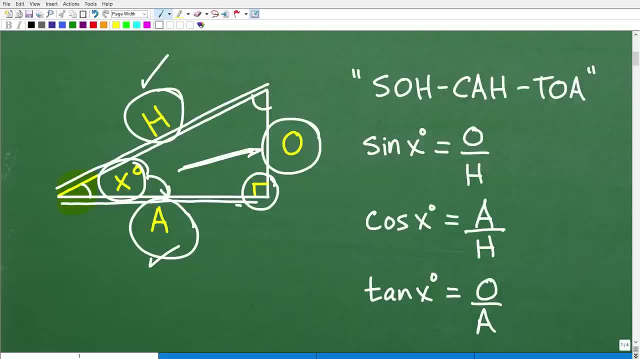 here. its adjacent side is this side here. its opposite side is way over here, and then this is always a hypotenuse. so let me go ahead and erase this now, and now we can actually be introduced to to some basic trigonometry, okay, so let me just erase this here so we can get nice. 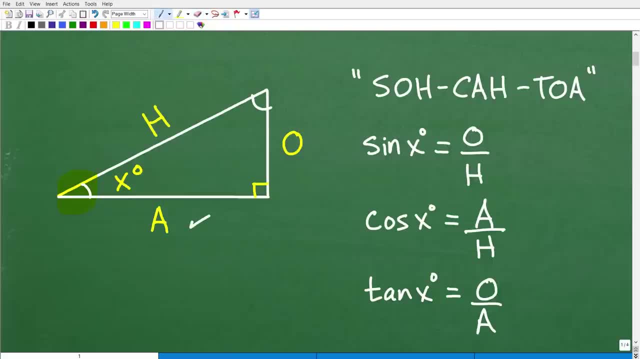 and focused. all right, so again we have the adjacent, the opposite and the hypotenuse. now let's go ahead and take a look at this little lovely saying right here now. if you've never seen this saying or if you never have heard this, uh, this is your first time. well, i could tell you. 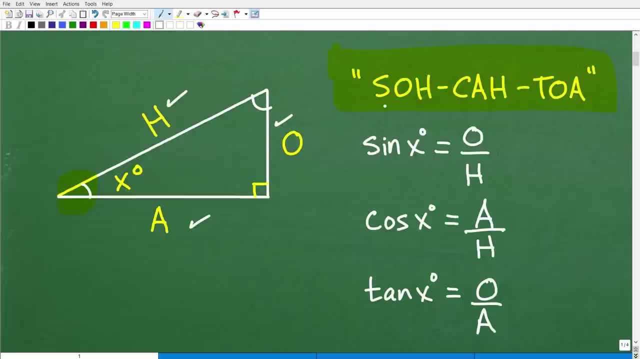 this saying has been around for decades. probably your great great grandparents even learned it. but here it is. it's called so katoa, so katoa, and a lot of you are like, oh my goodness, what this is? you know? it seems like a foreign language. well, it this is not. it's just a little helpful. 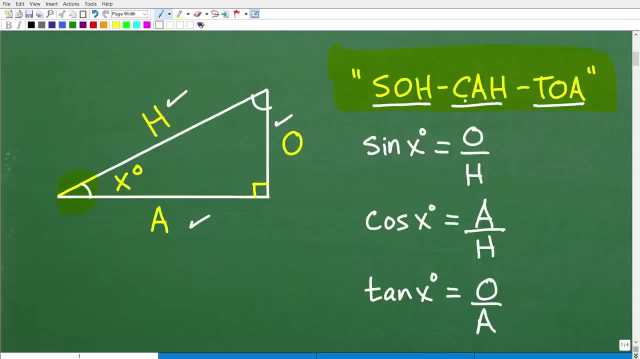 memory device, a mnemonic, we call it so. so, katoa, what does it stand for? well, let's start off with the s o h. so in trigonometry, in basic trigonometry, we have these uh things called trigonometric functions. so if you have a scientific calculator, you'll see these buttons here, you'll see a sign that's not a. 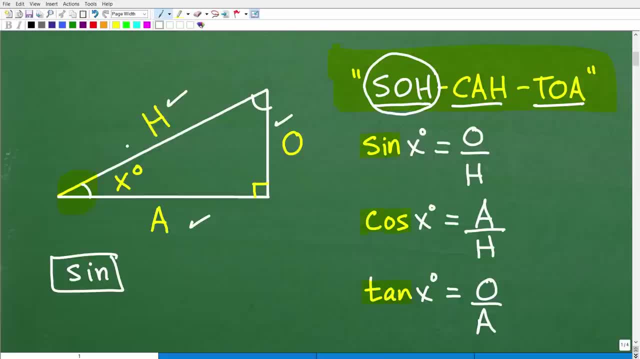 sin. okay, like: oh, this is, you're committing the sin by doing math. no, that's not what that means. this is called the sign. then we have the trigonometric function, and then we have the something called the cosine, and then we have this other thing over here called the tangent. 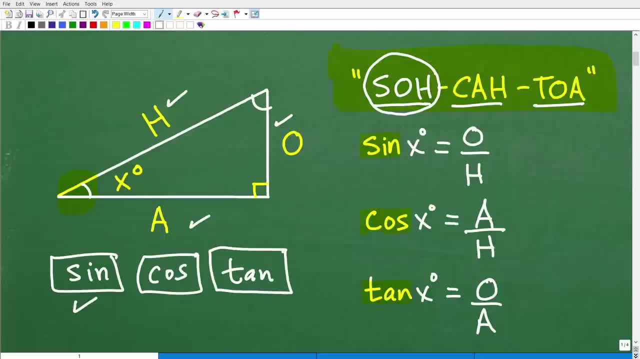 so if you have a scientific calculator, you'll find these buttons on your calculator. you need access to a basic scientific calculator if you're using your cell phone. generally, the calculators on a cell phone, typically on a smartphone, will have like, or just like, more basic functions. 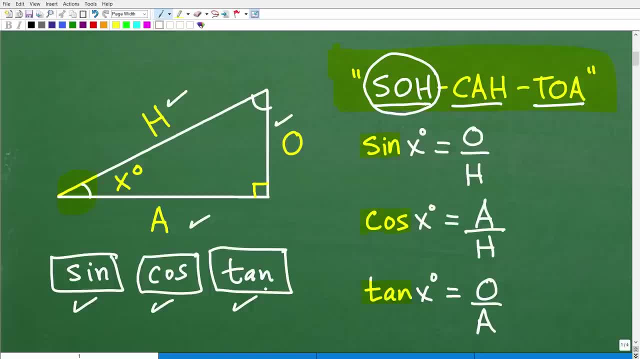 in like the basic number operations, so you'll have to kind of switch it to a different mode in order to get these. but you make sure you have access to the calculator and then you'll have to switch it to a calculator, whether it be on your calculator. i start on your phone and i do not. 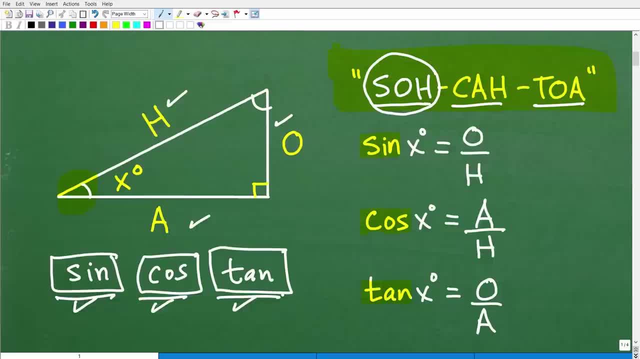 recommend you using your phone to study mathematics, because you're not going to use it, you're not going to be able to use it on a test. most teachers won't allow that. so get yourself a basic scientific calculator. it costs you all about 10 bucks at cvs or walmart and we're not talking about a graphing. 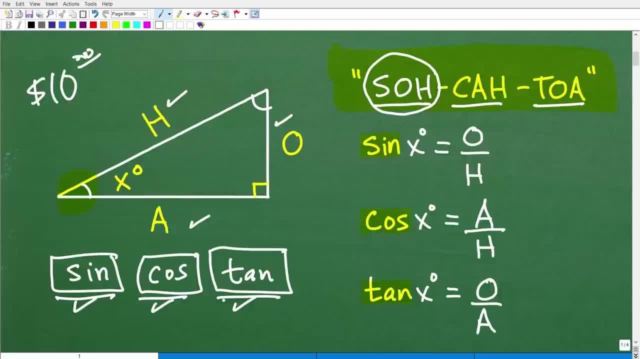 calculator. we're just talking about a scientific calculator that has these functions right here: sine, cosine and tangent and other functions anyways. so these are our basic trigonometric functions. so let's get back to this saying so, katoa, so the sine, okay, is defined as the opposite over the hypotenuse, okay, so the sine of this, 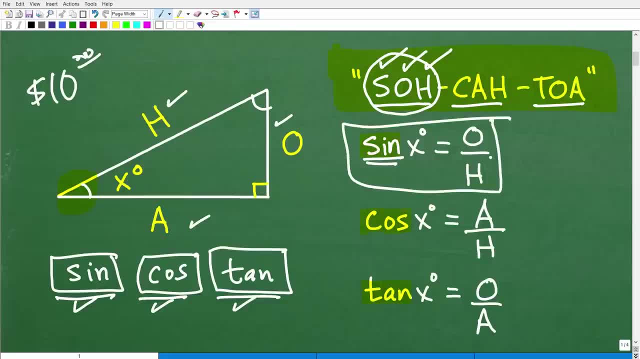 angle. right, there is the opposite over the hypotenuse. so we just kind of put that abbreviation sine- opposite over hypotenuse, or that's is the so. okay, so sine is equal to opposite over hypotenuse. that's how we remember it. cosine is adjacent over hypotenuse. okay, so that's so. 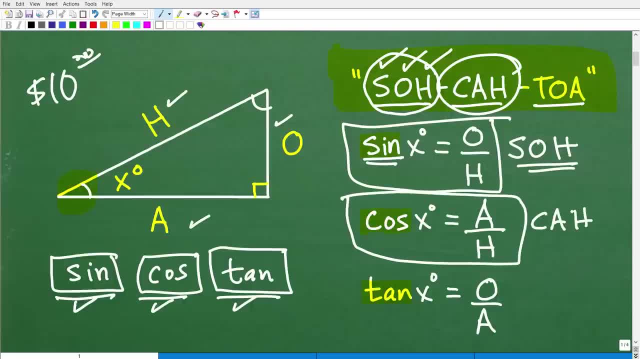 ka. so again, this is the ka. the cosine is adjacent over hypotenuse. and then we have this last one here, the tangent, which is the opposite over the adjacent. okay, so that is the tangent opposite over adjacent. so these are the basic definitions of these trigonometric functions. now there are other functions, but these are the ones that you really 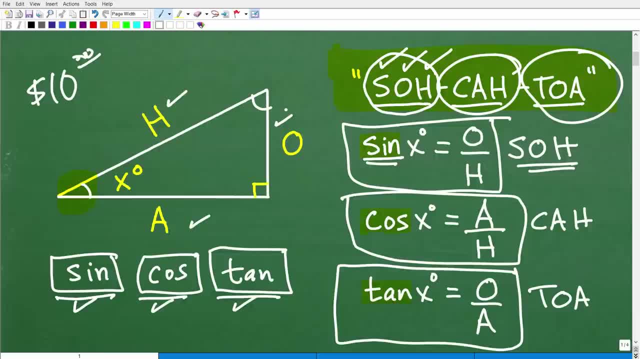 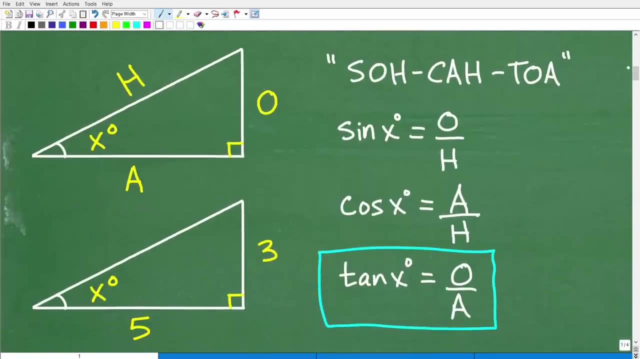 need and you can solve any right triangle trigonometry problem using these functions. okay, all right, so that's all this is here. so katoa, and that's the definition of these functions, but now let's go ahead and match this up to the problem. all right, so? 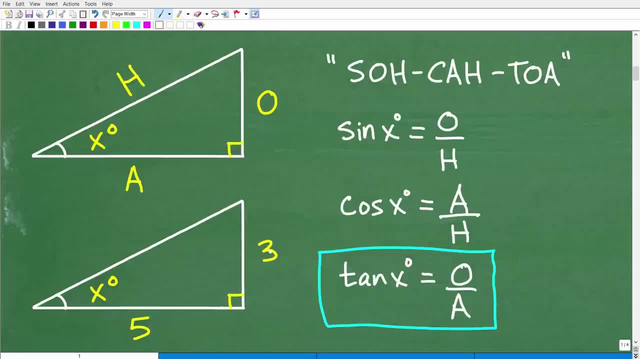 looking at this, here is our triangle, we have three and we have five and we're looking for for this angle right there. so three and five happen to be in what uh spots. in other words, three is the what side in terms of angle x and five is the what side. well, let's just go back to 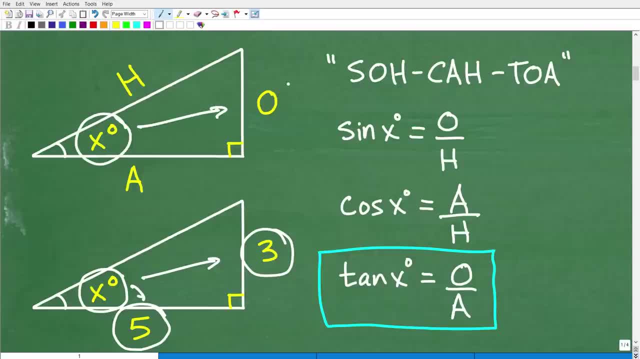 our basic right triangle. here's angle x. so three is the opposite side and five is the adjacent side. so the information we have for this particular triangle is the opposite and the adjacent. so now, when you think about that you're you go over to your silica toe and you'll be like, okay, which one has o and h? because that's what. 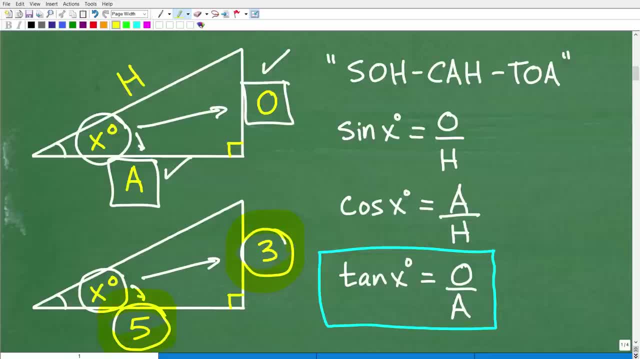 i have here. i have the opposite length and the adjacent length of this triangle. so i'm looking for something here which function has that involves both o and h. so i'm like, oh, this is, i'm sorry, o and a, excuse me, not o and ho and a. so i'm like, okay, this is o and h, this is a. 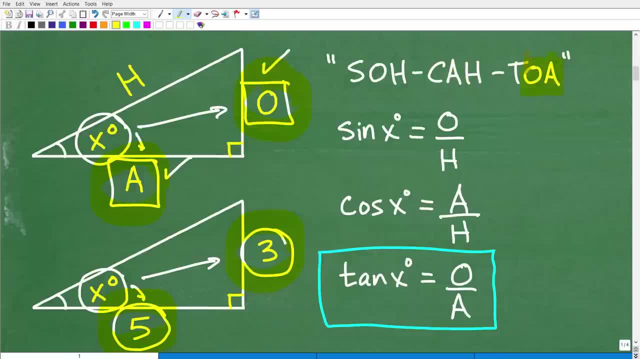 and h. this is not what i need. oh, i have the and the adjacent, so we're talking about the tangent. okay, so the tangent involves both the opposite and the adjacent. I apologize for saying hypotenuse there, but anyways, hopefully you'll understand that we have a choice. we can try to use the sine cosine or tangent, but the way we kind of 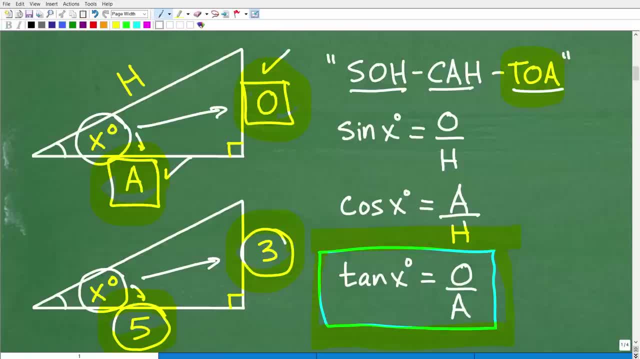 determine which of these functions that we're going to use is based upon the information given in the problem. so you're like: oh, I have the opposite and I have the adjacent, so I'm going to use the tangent to solve for this angle. all right, so now let's go ahead and see how this is done. 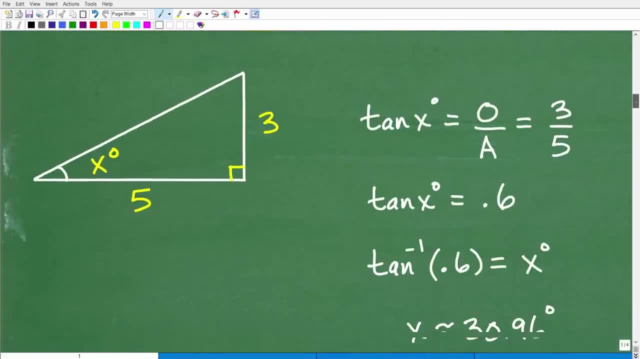 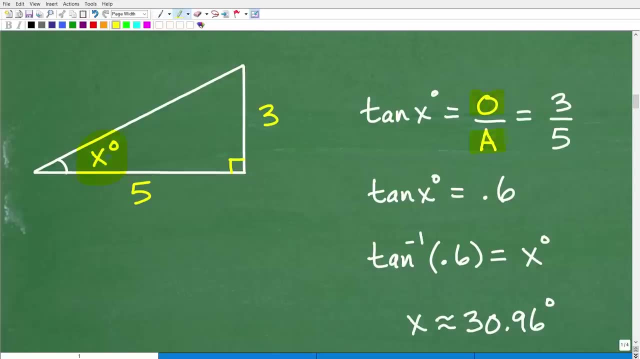 okay, so now, of course, we know that we're going to be using the tangent, so let's go ahead and define. the tangent of this angle right here, of course, is going to be the opposite over the adjacent. the opposite is three and the adjacent side is five. so the tangent, 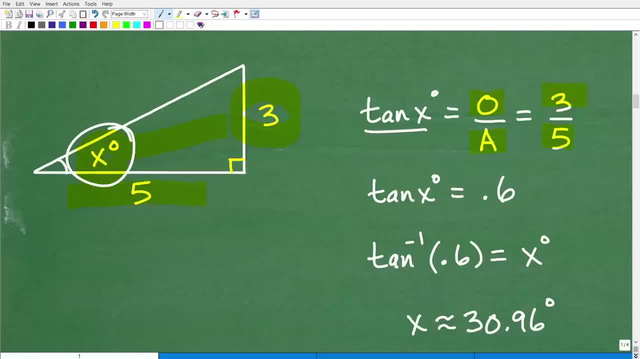 of this angle here, tangent of x degrees. we don't know how many degrees this is, but we do know it's equal to three over five or the opposite over the adjacent. now, three divided by five is 0.6. so the tangent of this angle- right there, okay, the tangent of x degrees is equal to. 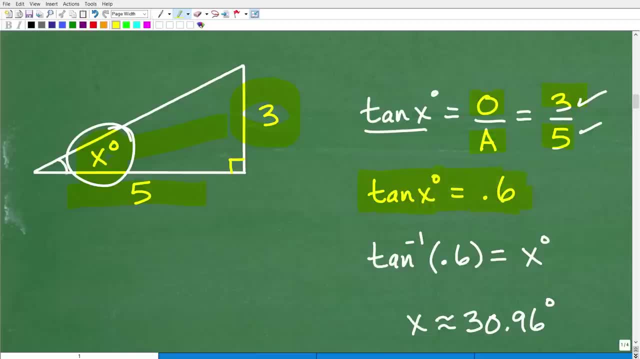 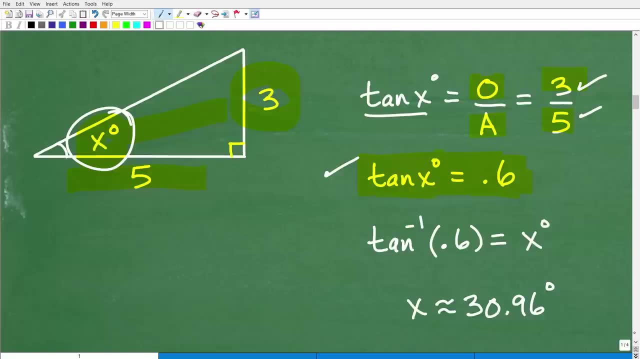 0.6 or three divided by five. so this is where we're at right now in this stage of the game. so at this point we're like, okay, how do we actually find the angle? well, in our calculator, okay, on your scientific calculator, when you have these buttons, tangent, sine and cosine, what you have is, if you look on that, 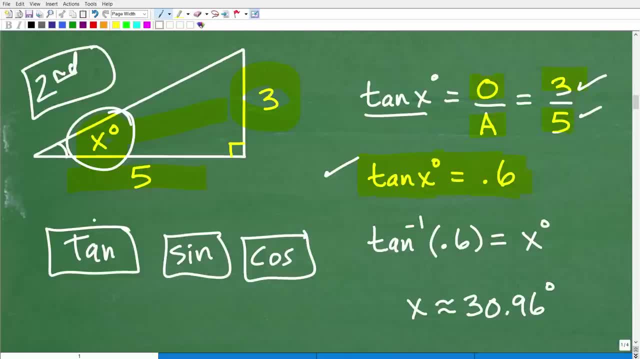 second function, and it's usually right on the kind of keyboard itself, you'll see this little actually write this in a different color. this is important. you'll see this function here: tan looks like a little negative one, and then sine like a little negative one and cosine like a negative one. these are called. 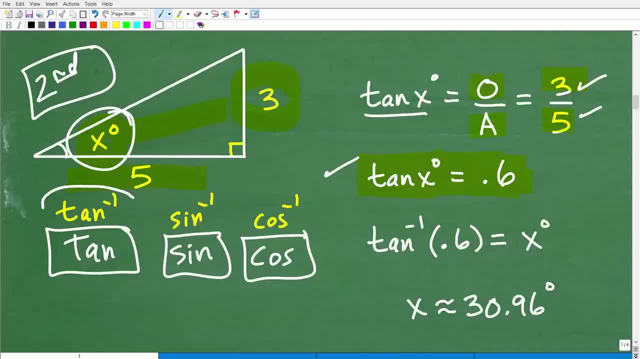 arc tangent, arc sine, arc cosine. we actually need these functions right here. so because we're dealing with the tangent, we're going to need this one, so we're going to have to use the second and tangent key to bring up this function. okay, so this function here. 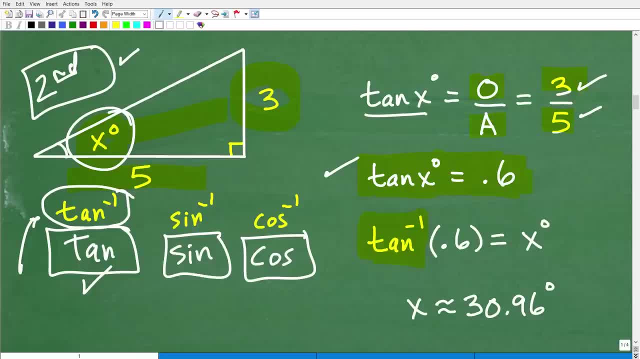 the arc tangent will tell us, if we say, hey, we have an angle, we know the angle, we have some angle, but we know that the tangent of that angle is 0.6. what is the angle? okay, so i'll say this again: we have some angle, we don't know what it is, we just know that the tangent of 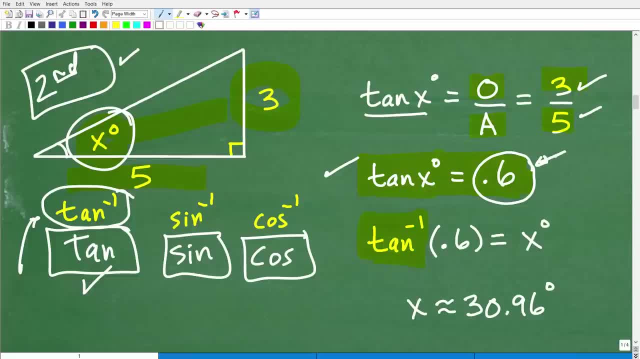 that angle is 0.6. how do we find the angle? because that's what we want to do here. well, you bring up this arc function, okay, this arc tangent, so that's going to be tangent negative one, and we plug in 0.6. this is basically saying, hey, tell me the angle. 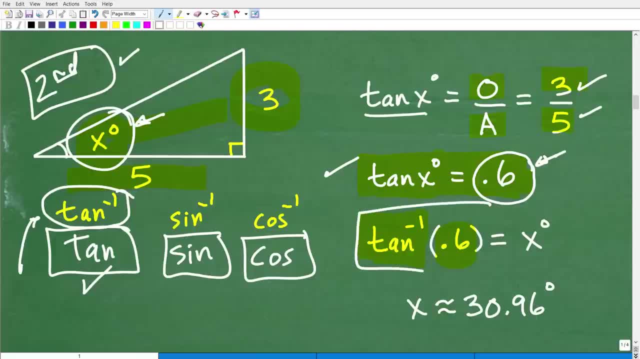 that has a tangent of 0.6. so when you plug this into your calculator- all right, this arc tangent is tan negative one- you'll see that little negative one there- 0.6- and you hit enter- okay, that's going to tell you the actual angle. okay, now the angle here is going to be approximately: 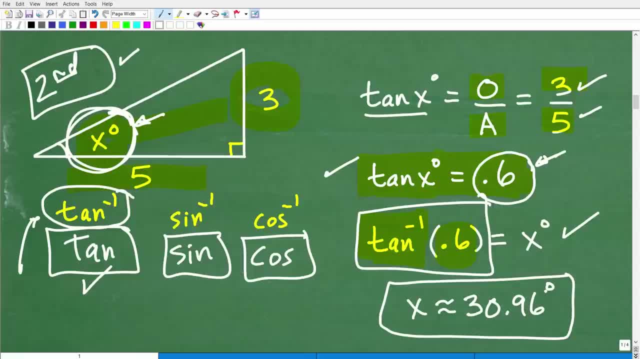 30.96 degrees. that is the answer. now let me just um stress something to you. uh, that gets a lot of students in trouble when they're when they start messing with trigonometry on your calculator. there is, in the mode part of your calculator, ways that we can work with different angle measures. there's basically two primary ones. 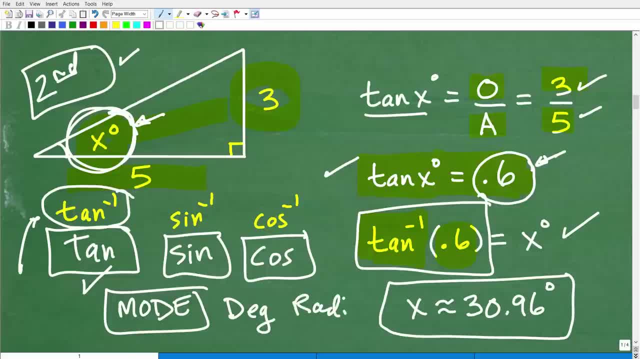 uh, one is the degrees and the other one is radiance. okay, the default setting for all calculators is going to be degrees. okay, so just make sure on your scientific calculator you see deg okay when you're doing this work, because if you see rad you will get the incorrect answer. 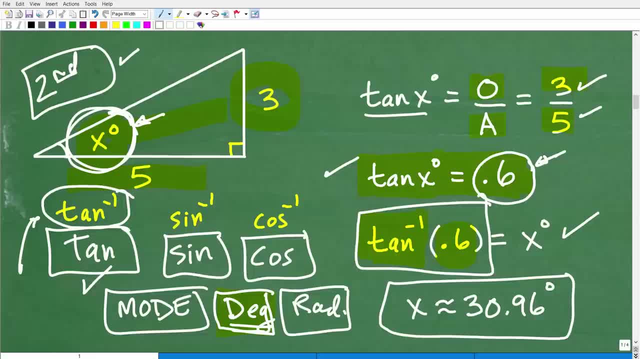 okay, a lot of students, when they're studying trigonometry and they have to work with radiance, forget to put their calculator back in degree mode and then they get in trouble like that. but as long as you're not messing with that mode, just most calculators by default are going to be in. 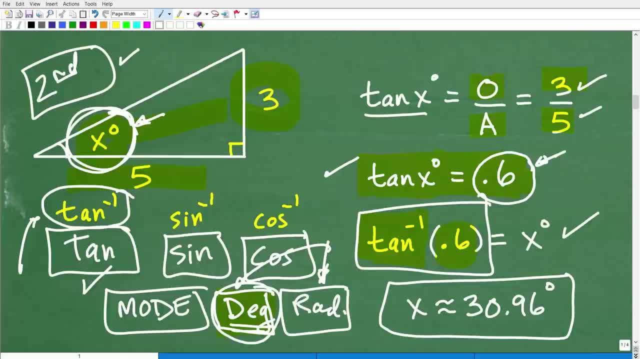 degree mode. okay, and this is not a trivial, a trivial little detail, as this does get a lot of students in trouble. so to make sure your calculator is in degrees, because we're trying to find out the angle measure here in degrees. that's what this little round circle up there is. so again, uh. 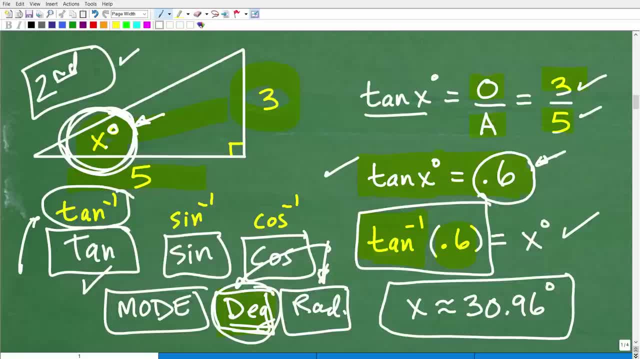 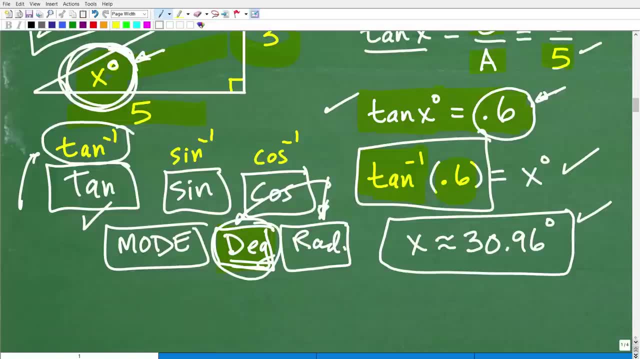 it's going to be. of course, i'm rounding off here, but the angle here, angle x, is going to be approximately 30.96 degrees. that is the answer. okay, so how did you do? did you actually do this on your own? i mean, if you knew how to do this already, i must go ahead and give you a nice little. 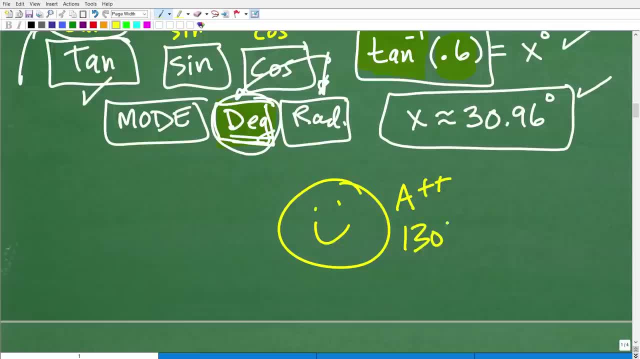 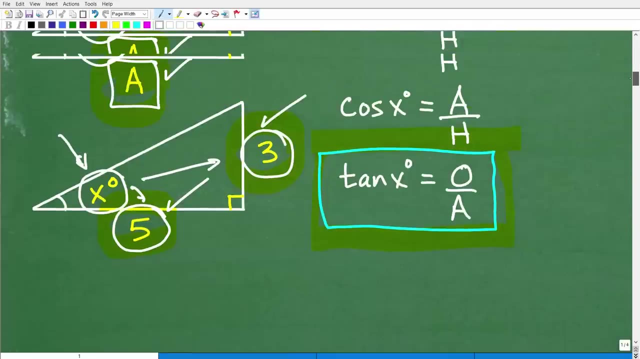 lovely, happy face, an a plus plus at 130 percent and multiple stars, because you are pretty awesome knowing, um, some basic right angle trigonometry. now let's go back to uh, this setup right over here. okay, so here we decided that we were going to use the tangent. 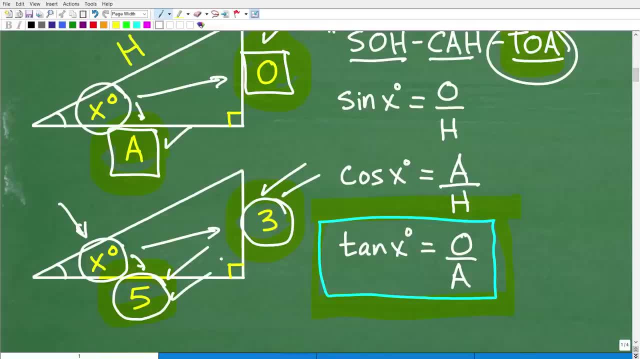 because we had the opposite and the adjacent side. now, if i was uh, so inclined, i could have used the pythagorean theorem: a squared plus b squared is equal to c squared. okay, to solve and get the hypotenuse and get the h value right there. okay, i could have easily done that. and once i had the 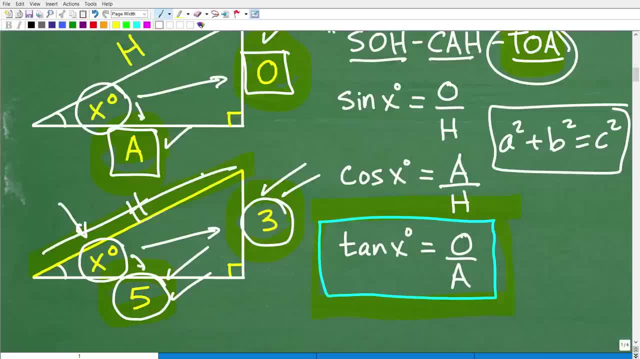 hypotenuse. i could use these other functions like cosine or sine to get the same answer. but again, that's not necessary. as long as you have two pieces of information in a right triangle, just use whatever particular function that goes with. uh, the problem right. so here i have again the 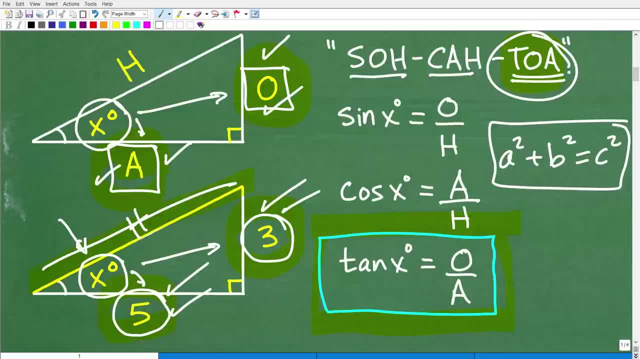 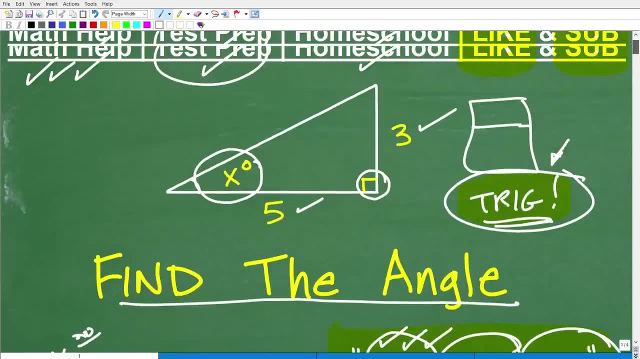 opposite and the adjacent. that uh led me to be like: oh, i must use the tangent, not the sine or cosine. but if this is your first introduction to trigonometry- well, hopefully it was an exciting one- you can see that there's no other way i can solve for this angle. 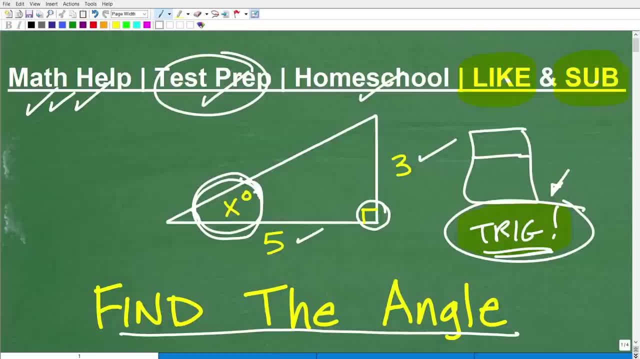 here without using basic right angle trigonometry. this is the whole value of learning trigonometry. and again, this is an introduction to trigonometry. trigonometry is much, much more advanced. so a couple suggestions here. if you want to know more about trigonometry, i have additional videos.